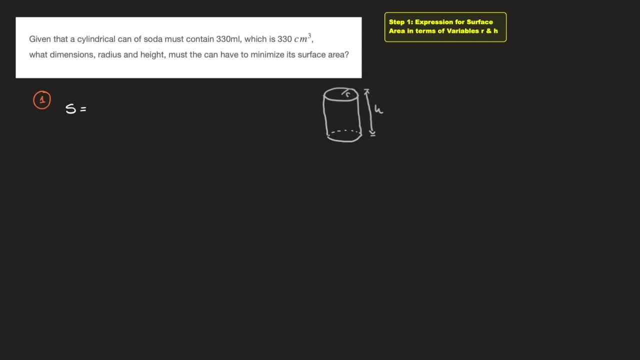 surface area s, then it's going to equal to the surface area of the disk at the top plus the surface area of the disk at the bottom. So I'll start by just drawing those. I have a disk at the top plus a disk at the bottom, And alongside that we have the curved surface area. 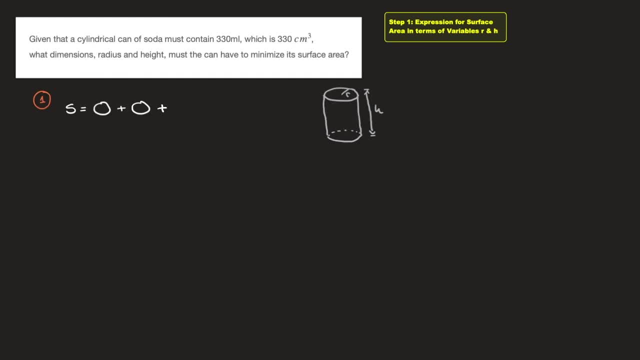 wrapping itself around the can. Now, that surface area is, in fact, a rectangle which wraps itself all the way around the cylinder, And what that tells us is that the base of this rectangle has to equal to the circumference of the disk at the top and at the bottom, And that circumference is equal to 2 pi. 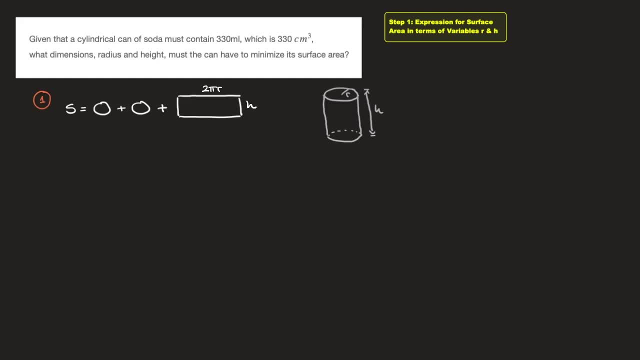 r, The height of the rectangle is h, And each of the disks here have a radius of r. All right, now that we've made all these sketches to help us, let's go ahead and write this all in mathematical notation. The area of each disk is pi r squared, So we have pi r squared plus. 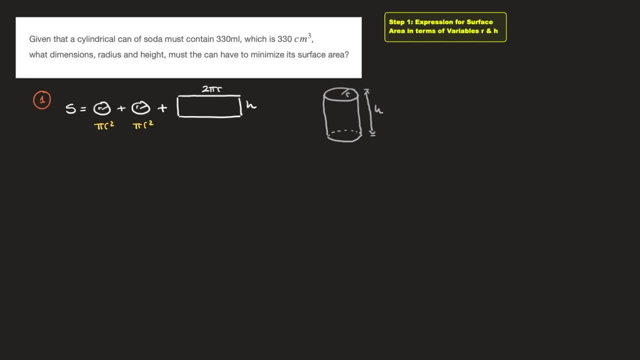 pi r squared And the area of this rectangle is base times height. So that's 2 pi r times h. Finally, since pi r squared plus pi r squared is 2 pi r squared, we can go ahead and state that the surface area s is equal to 2 pi r squared plus 2 pi r times h. And that's our first step. 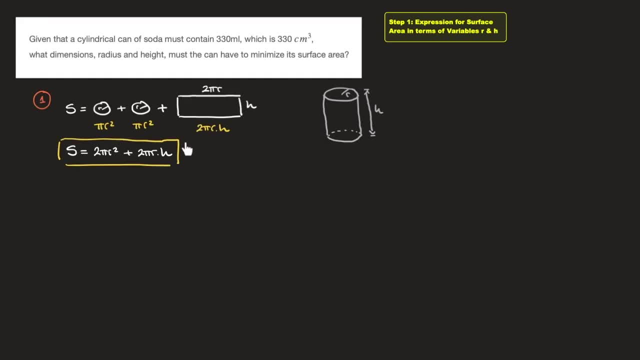 done. We now have an expression for the quantity we're trying to optimize, in this case the area of the disk at the top of the cylinder that we can call the surface area. it's the surface area we're trying to minimize, written in terms of the. 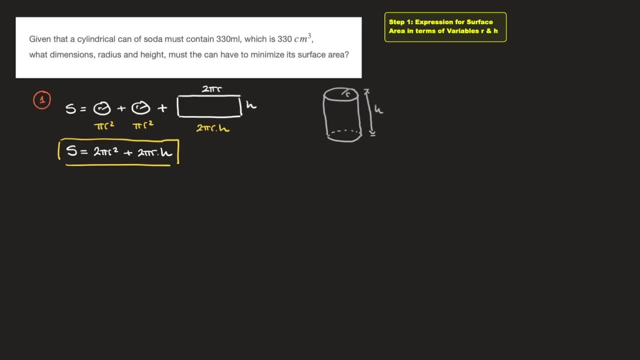 variables we have, which are R and H. so we move on to step 2 and in step 2 we need to find or identify the constraint and write it in terms of the same variables as we did in step 1, so those would be R and H. now, when I say 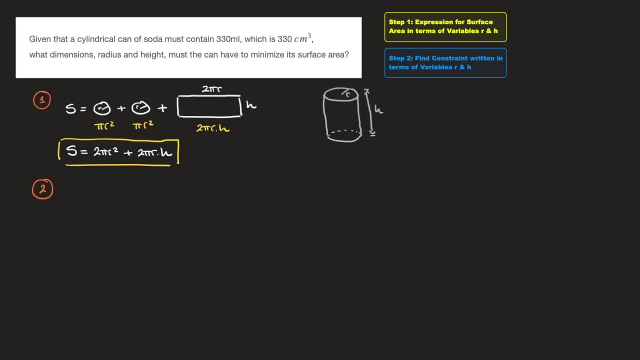 constraint. you can think of it as what's the limitation? and in this case we're trying to minimize the surface area. so when I say limitation, ask yourself what's stopping us from making the surface area equal to zero? and as we read through the question again, we quickly see that the only limitation 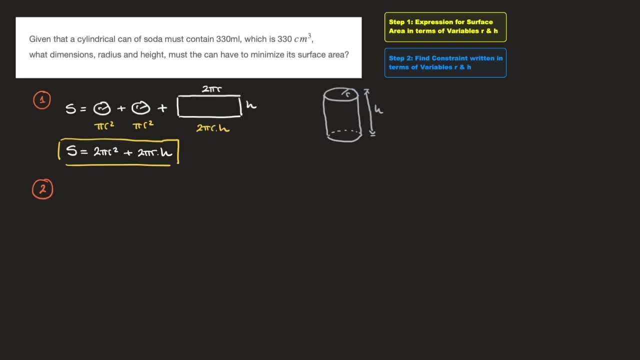 we're dealing with here is the fact that the volume of the cylinder must equal to 330 cubic centimeters. so the constraint or limitation is the fact that the volume, which I'll go ahead and call V- has to be equal to 330. and so now that 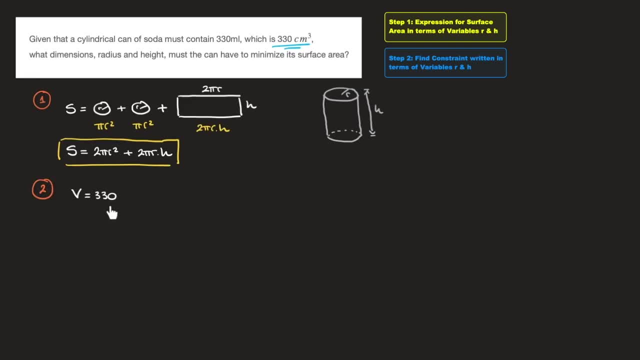 we've identified this constraint, we need to write it in terms of the variables H and are, and for that we use the fact that the volume of a cylinder is equal to the area of the disc at the base, so that's pi R squared times the height of. 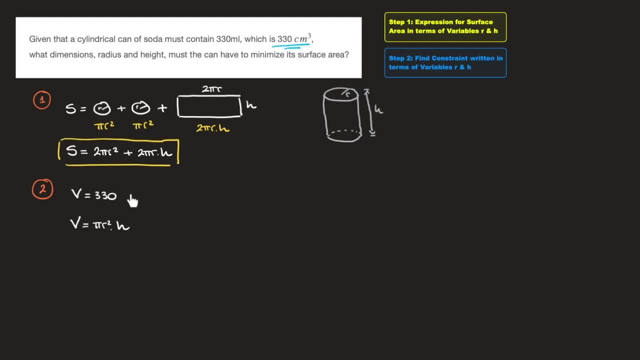 the cylinder, which is just H, and combining these two results, we quickly find that the constraint is the fact that pi R squared times H must equal to 330, and that's our second step done. we now have an expression for the constraint written in terms of the variables R and H, so we move on to step. 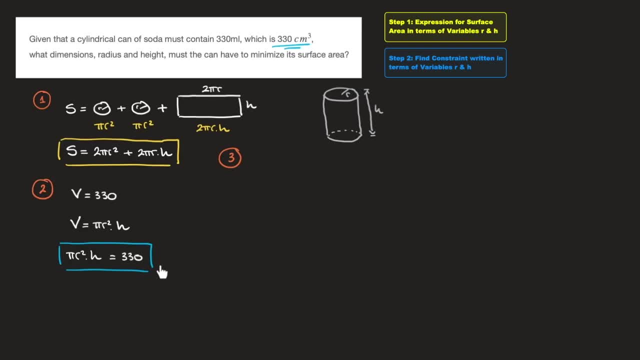 three, and in this step we need to use the expression for the constraint we just found to eliminate one of the variables, so R or H, inside the expression for s, the objective being to only have one variable left inside our expression for the surface area. so let's see, starting from our constraints, so that's pi R squared times. 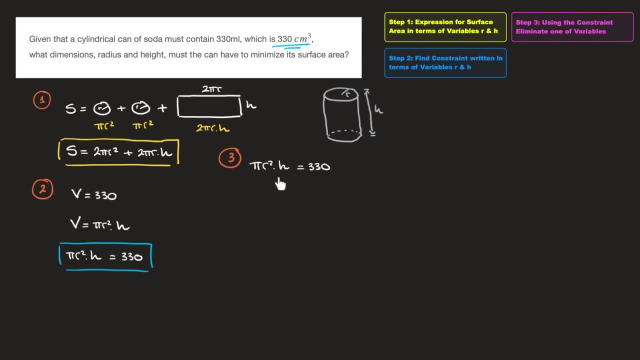 H, which equals to 330. we can rearrange this to make either H or R the subject. looking at this, it seems easiest to make H the subject. indeed, for that, all I have to do is divide both sides by pi, R squared. in other words, I can quickly. 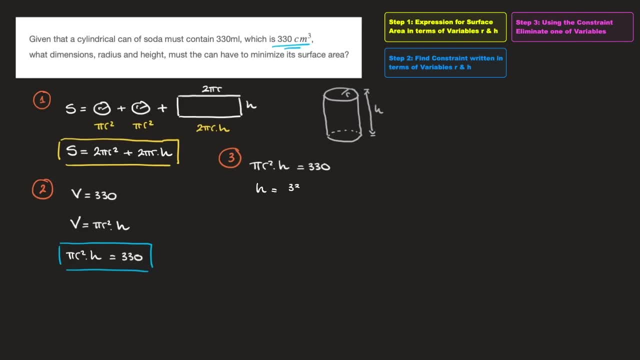 rearrange this: to write H equals to 330 over pi R squared, and I'll go ahead and box that in blue just to remind us that we obtained that from the constraint. and now that I've done that, I can go back to the expression I have for s here and replace every H. I see so this: 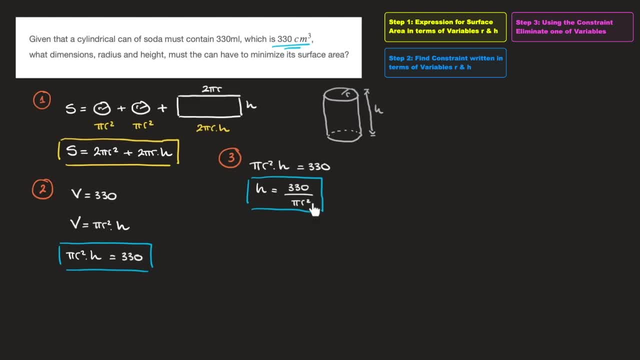 one here by 330 over pi R squared, and that will eliminate the H. so that would be: s equals to 2 pi R squared plus 2 pi R times 330 over pi R squared. now, multiplying this new numerator by 2 pi R leads to 2 pi R squared plus 660 pi R over pi R squared. 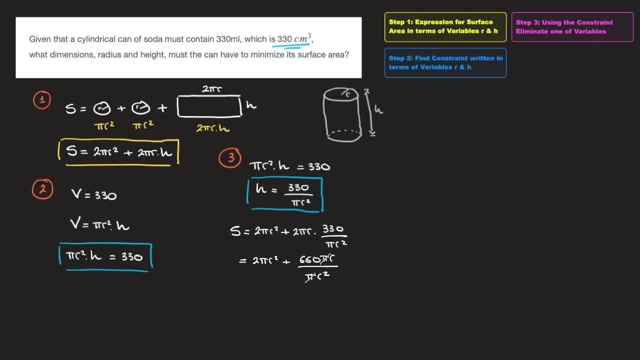 and now simplifying this pi on the numerator and denominator, as well as this R, and this R squared leaves us with s, is equal to 2 pi R squared plus 660 over R, and that's the third step done. we now have an expression for the quantity we wish to optimize. written. 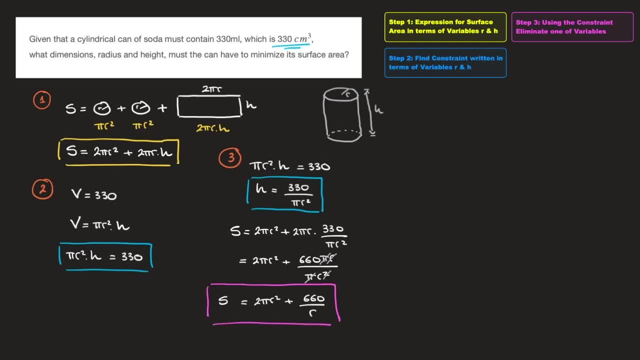 solely in terms of one of the two variables. and in fact, now that it's written this way, we could go ahead and specify that the surface area is written as a function of R only. so that's s of R. and now that's done, we move on to the 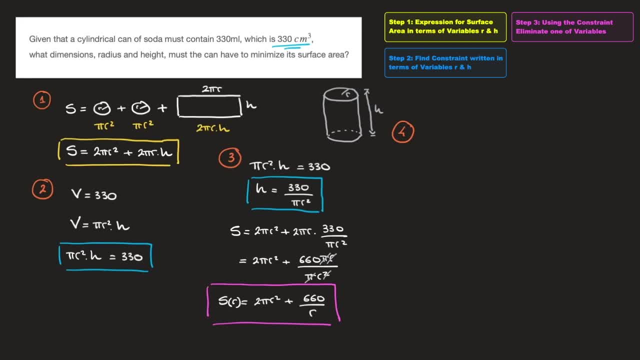 fourth and final step, and in this step we use calculus to optimize, or in this case, we use calculus to minimize, meaning find the minimum value of the surface area, which is this function here. So let's see, starting from the function s of r, which equals: 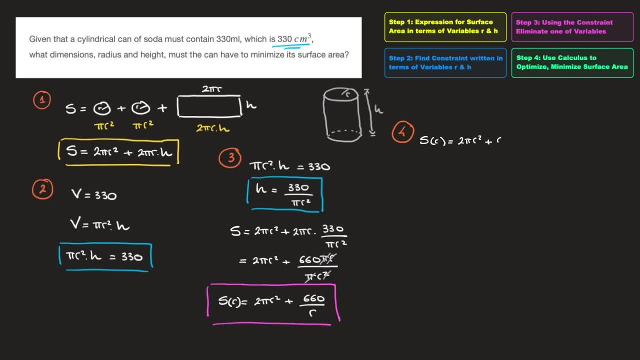 to 2 pi r squared plus 660 over r. the first thing we need to do is differentiate it, And for that I go ahead and use the power rule and state that s dash of r is equal to 4 pi r minus 660 over r. 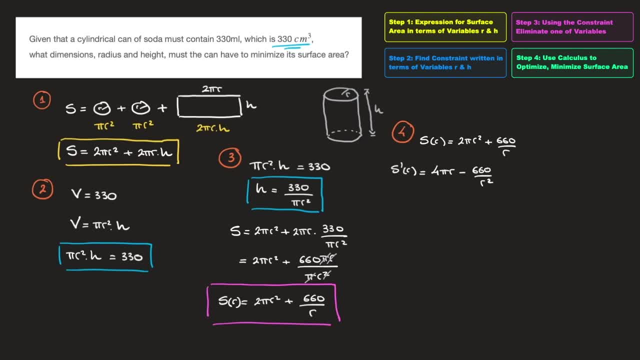 squared. And let me point out, I'm sure you have no trouble in seeing how I got from 2 pi r squared to 4 pi r as quickly. but if you're in any doubt as to how to get from 660 over r to negative 660, 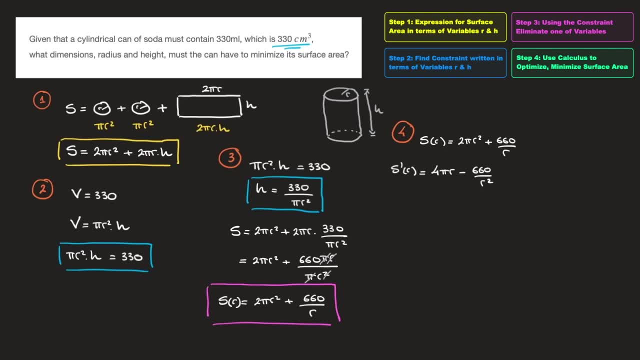 over r squared. let me just say that all I used is the fact that when we differentiate 1 over x, we'll always obtain negative 1 over x squared, And we could, of course, obtain this result by using the power rule, but knowing this result off by heart is definitely useful. 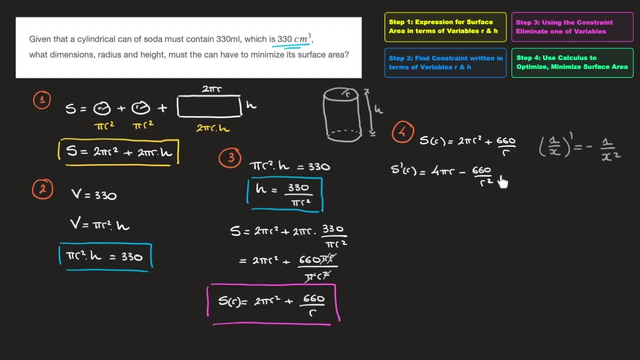 it comes up a lot. So that's what I used to get from here to here. All right, I now have the derivative and in fact I'll box that intermediate result. There we go, And so to find any minimum value our function s of r has, we need to equate this derivative to 0. In other words, we need to. 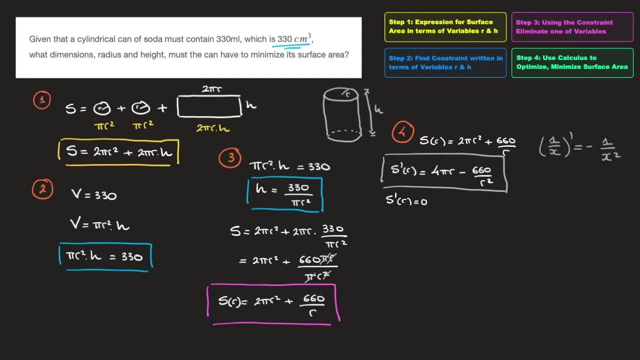 solve s dash of r equals to 0, which is the same thing, of course, as solving 4 pi. r minus 660 over r squared equals to 0.. Now, to solve this equation, I start by adding 660 over r squared to both sides of the equation. 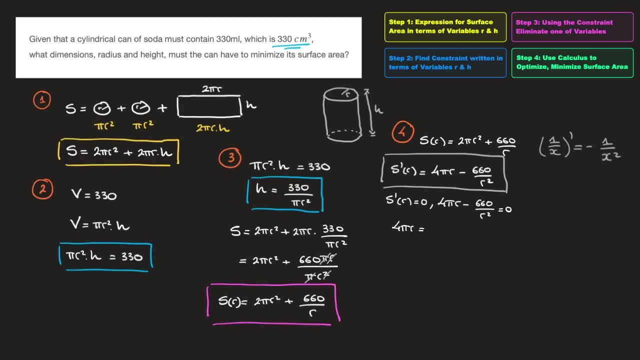 which leads us to 4 pi r equals to 660, over r squared. I now multiply both sides by r squared, which leads to 4 pi r cubed equals to 660.. I now divide both sides by 4 pi, which leads to. 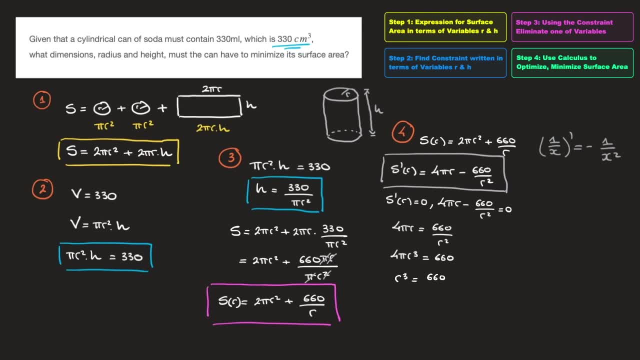 r cubed equals to 660, over 4 pi, which we can simplify to say that's equal to 165 over pi. And finally, taking the cubic root of both sides of this equation, we find that the radius r is equal to the cubic root. so that's the cubic root of 165 over pi. And by all means check, but with. 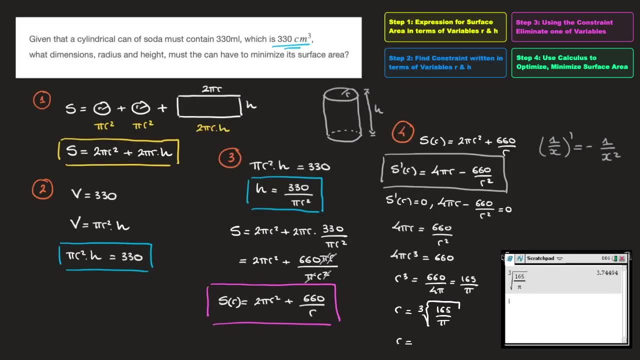 a calculator and rounding to two decimal places, I find that's equal to 3.74 centimeters. Done, Okay. so at this stage we know that the function s of r, and therefore the surface area, reaches a stationary point when r is equal to 3.74.. But how can we be sure that this indeed corresponds? 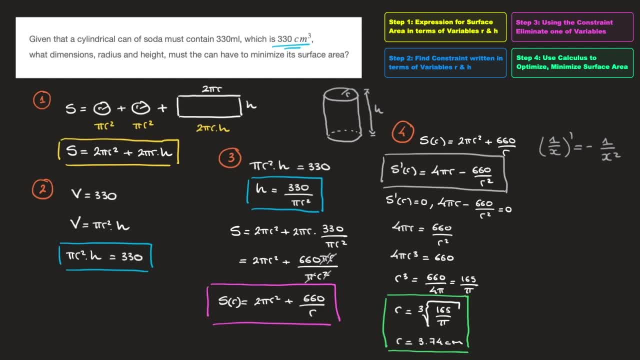 to a minimum value for the surface area. Well, one way of checking is to use the second derivative test, And for that the first thing I need to do is find an expression for the second derivative. So, starting from the first derivative, that's s dash of r, which I'll read out to you as well. 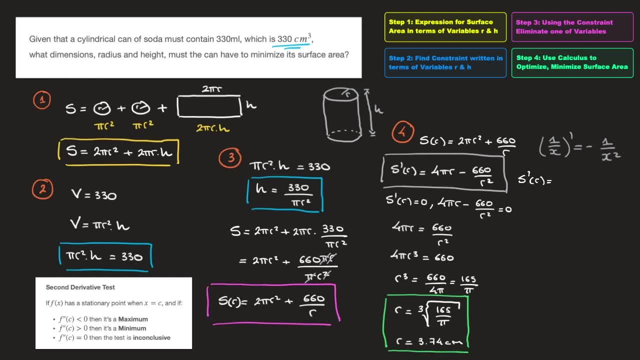 right here, as s dash of r equals to 4 pi. r minus 660 times r to the negative 2.. Notice here that to get this r squared away from the denominator, I added this negative power here. If I differentiate this again using the power rule, we obtain s dash dash of r equals to 4 pi minus negative 2 times. 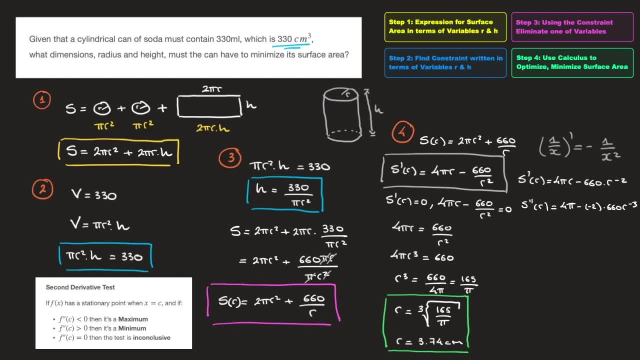 660 times r to the negative 3, and that's equal to 4 pi plus 2 times 660, which is 1320 times r to the negative 3.. In other words, the second derivative s dash dash of r is equal to 4 pi plus 1320 over. 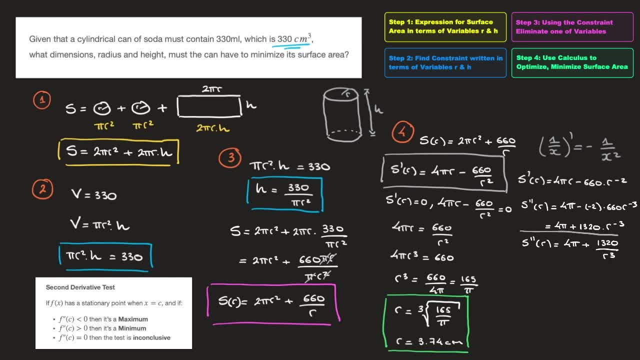 r cubed, and again, I could go ahead and box that intermediate result. There we go. Okay, now that we have the second derivative to determine whether our function s of r reaches a minimum when r equals to 3.74, all we have to do is evaluate this second derivative at this value of. 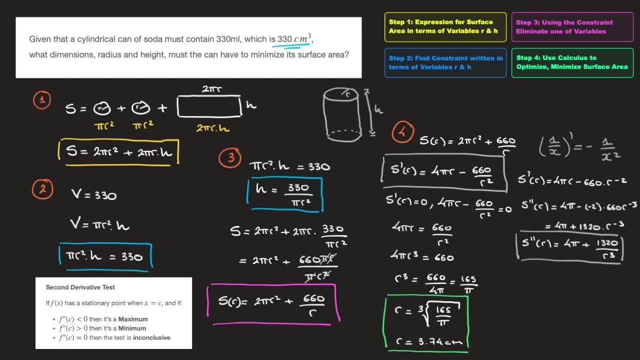 r and determine whether it's positive or negative. So let's see: if I replace r by the cubic root of 165 over pi, the second derivative s dash dash at the cubic root of 165 over pi is equal to 4. pi becomes 4 pi plus 1320 over the cubic root of 165 over pi cubed, which is just 165 over pi. Now I 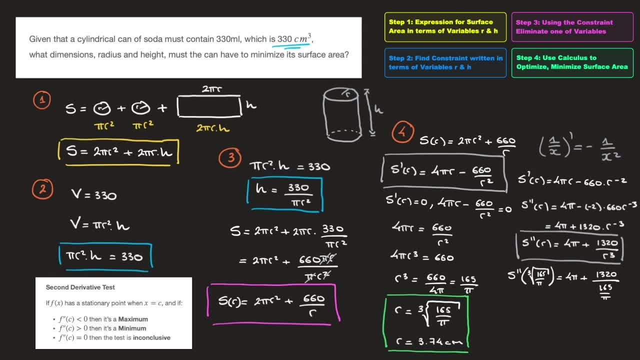 could, of course, go ahead and actually calculate all of this, but keep in mind, when we use the second derivative test, all we really care about is whether or not the result is positive or negative. and looking at all this well, it's quite clear that 4 pi is positive and 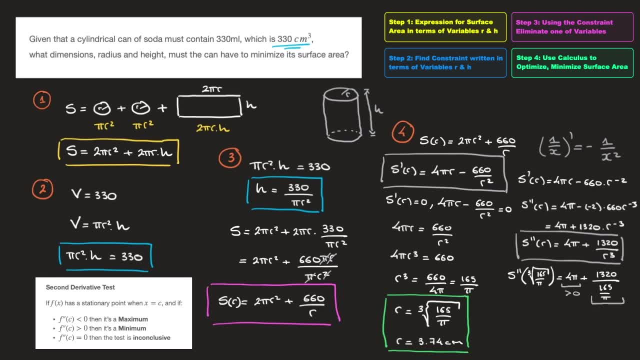 1320 over pi is equal to 4 pi plus 1320 over pi. 1320 over 165 over pi is also positive. Consequently, the second derivative at that value of r is positive, which allows us to conclude that our function s of r reaches a minimum value when r. 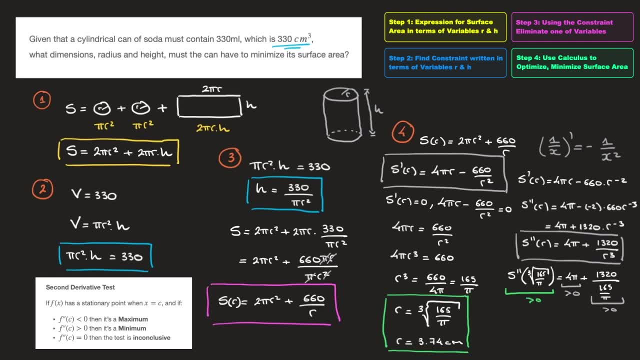 equals to the cubic root of 165 over pi. In other words, without even calculating, we can go ahead and state that we're dealing with a minimum. and now that that's established, all we have to do to finish this problem is calculate the height of the cylinder. 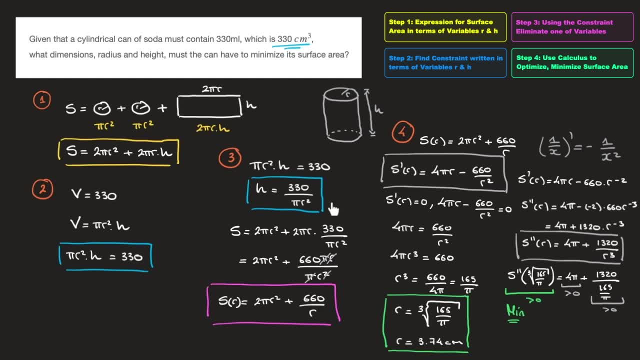 And for that we go back to the expression that I wrote here and replace r by the cubic root of 165 over pi. In other words, h is equal to 330 over pi, times in parentheses, the cubic root of 165 over pi, all of which is squared. 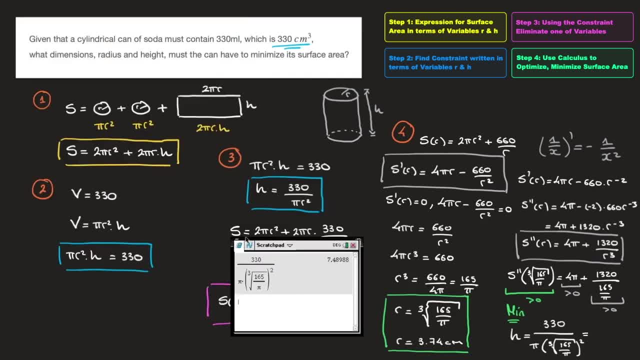 And by all means check, but with a calculator and rounding to two decimal places, I find that's equal to 7.49 centimeters and that's the final answer. we can now state that for this soda cans surface area to be minimized, its radius needs to equal to the cubic root of 165 over pi, or 3.74 centimeters, and its 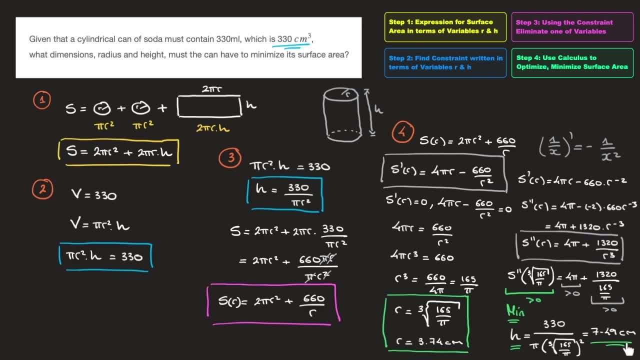 height needs to equal to 7.49 centimeters and, as such, we've now completed this problem. but, I should add, although we weren't asked to do it, we may well have been asked to do it in the future, So we're going to have to do it in the future. 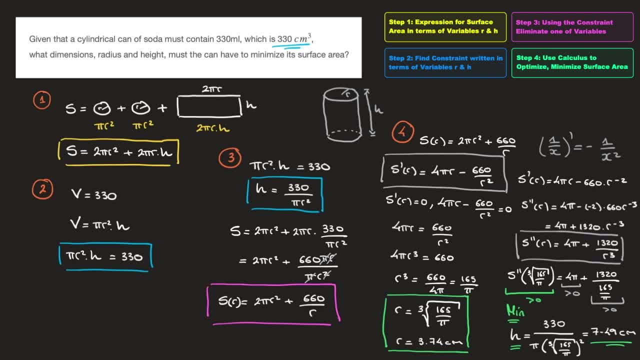 So we're going to have to do it in the future To actually calculate what the minimum surface area is, and had that been the case, all we would have to do is use the expression we have for the surface area here written in terms of R, and replace every R that we see by the 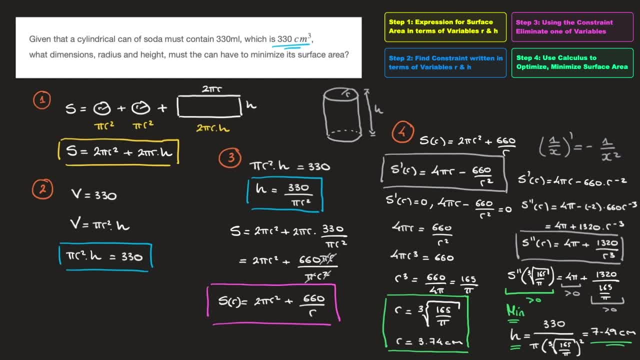 cubic root of 165 over pi, and in doing so using a calculator, we would find that the minimum surface area is two hundred and sixty four point three, five, seven square centimeters. and there we go. we now know how to answer this must know optimization problem. and that's it for this tutorial. 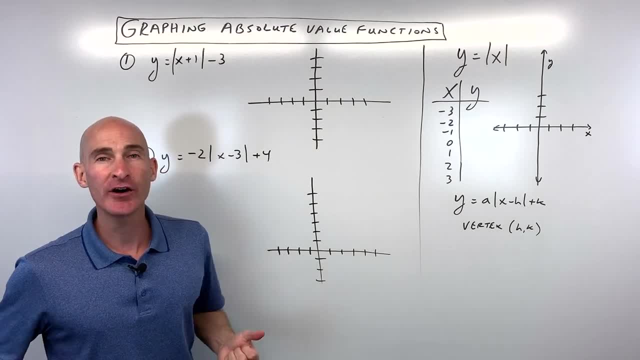 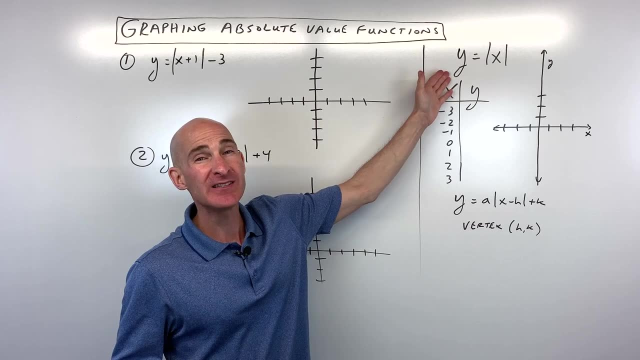 In this lesson you're going to learn how to graph absolute value functions with transformations. We're going to go through three examples, so let's dive in. The first thing you want to know is the basic shape of the parent function. this y equals absolute value of x. graph: 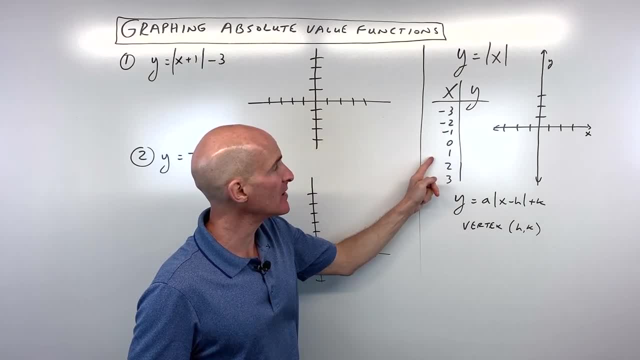 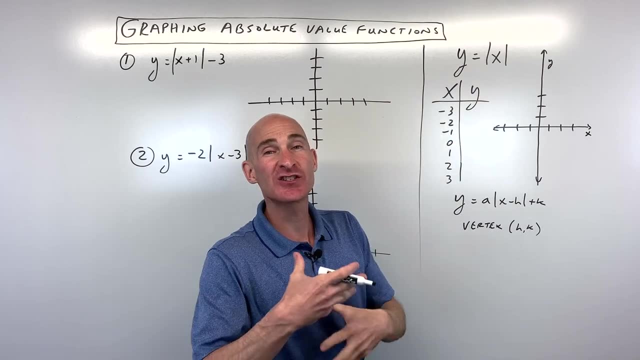 And the way you would get points for this graph is by picking a few negatives- zero and a few positives. So let's go ahead and do that. So negative 3, when we put it between these absolute value bars, that tells us to make the quantity positive.